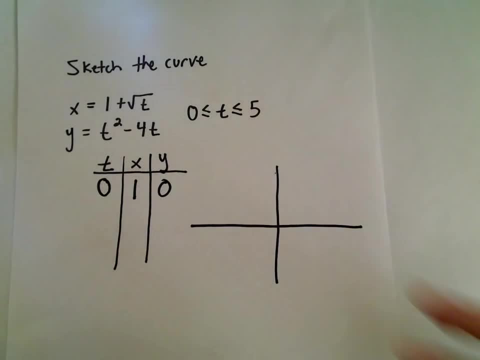 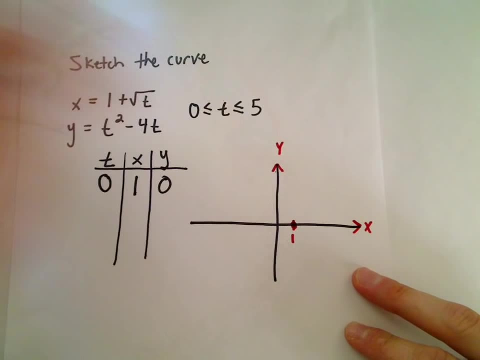 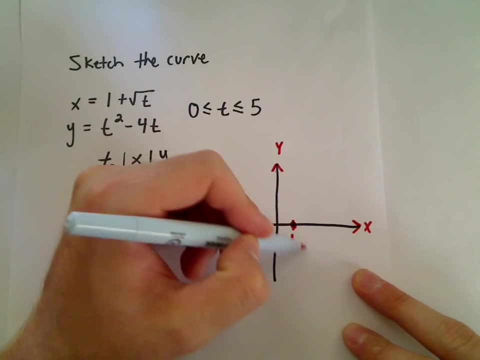 And what that means is: the point is on our graph. So here's our x-axis and our y-axis. So the point is on our graph And that corresponds to a t squared, So we have a t value of 0. This point, that corresponds to t equals 0, is what is called our initial point. 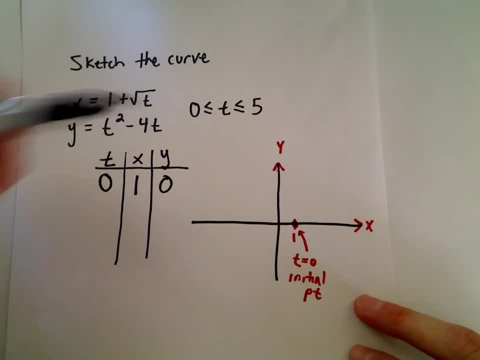 Okay, And now in this case, t can vary between values between 0 and 5, so let's plug in some other values. Maybe we'll plug in t equals 1.. If you plug in t equals 1, we'll get 1 plus 1, or an x coordinate of 2.. If we plug t equals 1 into the second and plug in t equals 1,, we'll get 1 plus 1, or an x coordinate of 2.. If we plug t equals 1 into the second and plug in t equals 1,, we'll get 1 plus 1, or an x coordinate of 2.. 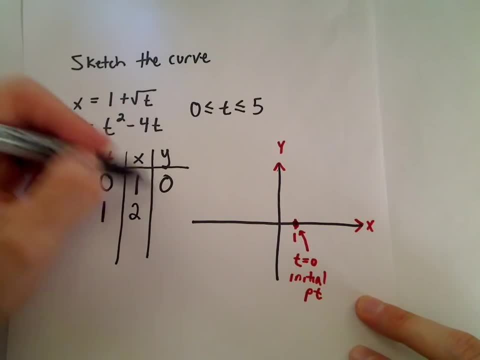 If we plug t equals 1 into our y value notice, we'll get 1 minus 4.. 1 minus 4 is negative 3. So that means the point is also going to be on our graph. I'm going to skip and then take a t value of 4, because that's easy to take the square root of. 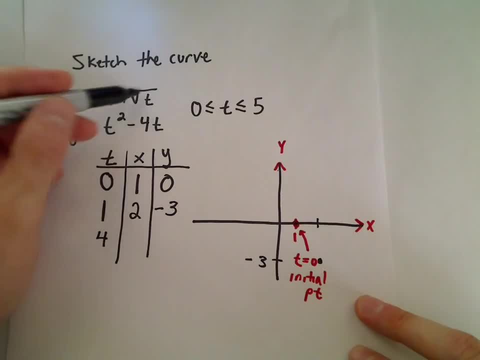 And we'll get, let's see, 1 plus square root of 4.. That's 1 plus 2, or an x coordinate of 3.. And then if we plug in our t value of 4, we'll get 4 squared, which is 16, minus 4 times 4, which is 16.. 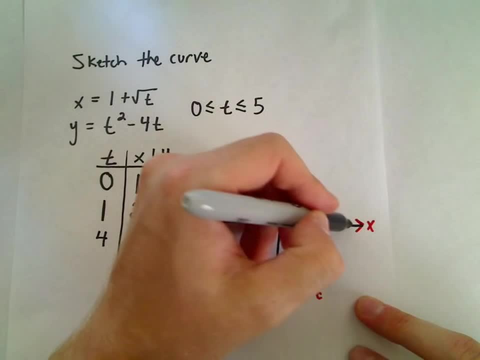 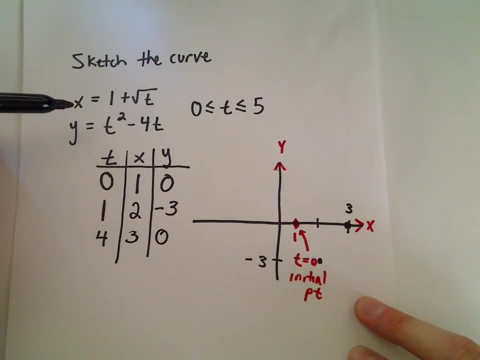 So we'll actually be back at 0.. So once we're at the x coordinate of 3, we'll be back at 0.. And notice as t progresses. that's what's going to happen. The x coordinate is going to get bigger. 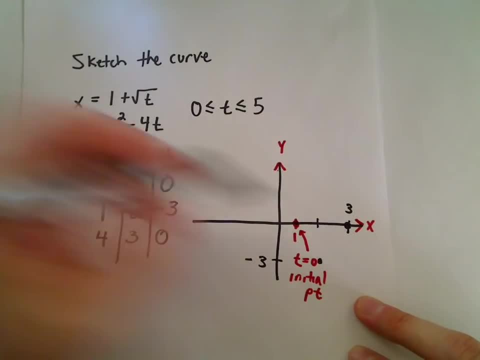 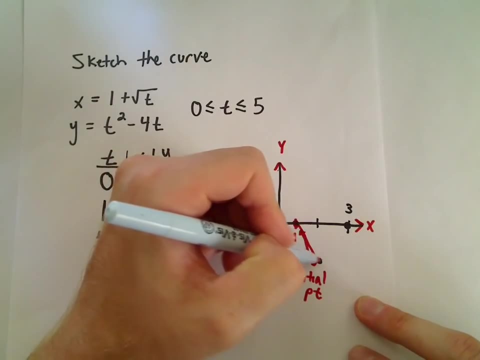 The y coordinate will get a little smaller, but eventually it'll start getting bigger as well. So here's our curve. I don't know, we'll just play, connect the dots, We'll assume we don't really know the shape of it. 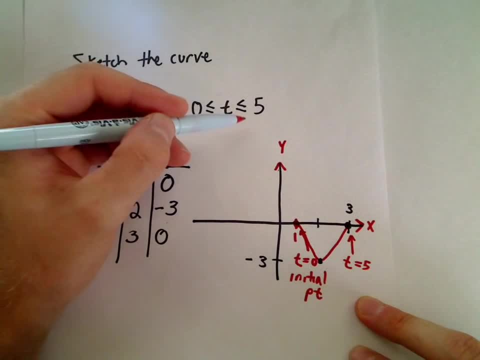 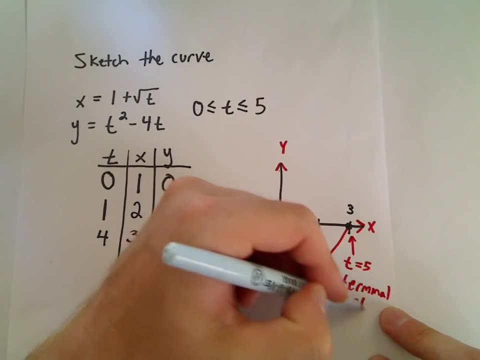 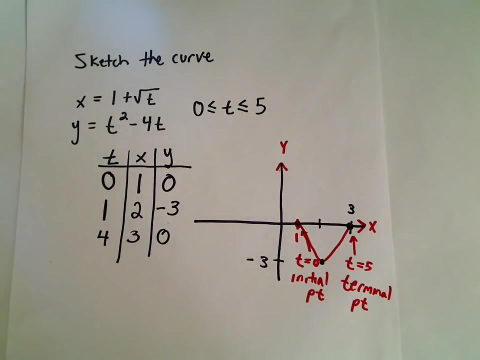 This point that corresponds to t, equals 5, in this case, since t is between 0 and 5, that's what's called the terminal point. Okay, so maybe let's just sketch a couple other ones here too, just to get a basic feel for what's going on. 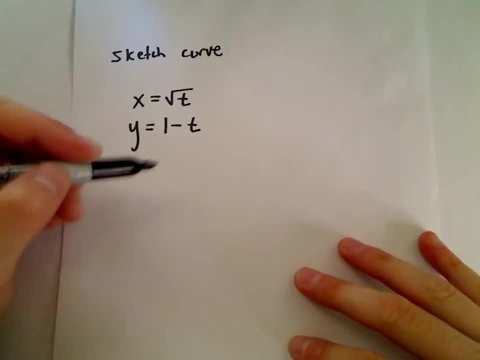 Suppose in this case we have that x equals square root of 4.. So we'll take square root of t and y equals 1 minus t. So in this case we'll pick values for t, x and y Again. maybe I'll plug in values that are easy to take the square root of 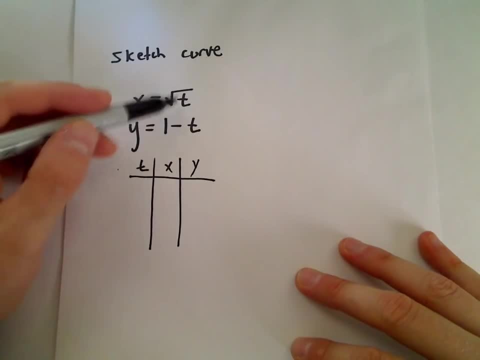 Notice here, there's no restrictions on t that are given, but of course t has to be greater than or equal to 0, since it's underneath the square root. So maybe we'll use 0,, 1,, 4, and then 9 just to see what's going on. 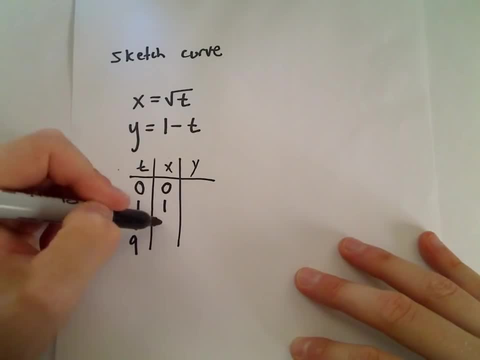 So square root of 0 is 0.. Square root of 1 is 1.. Square root of 4 is 2.. Square root of 9 is 3.. And then 1 minus 0 is 1.. 1 minus 1 is 0.. 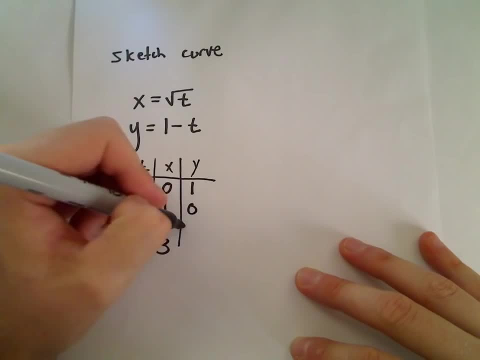 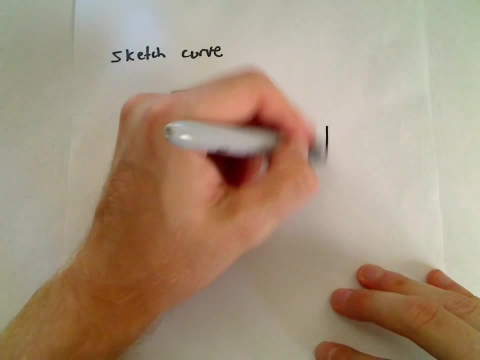 If we plug t equals 4,, we'll get 1 minus 4, or negative 3.. If we plug in 9,, we'll get 1 minus 9, or negative 8.. So now I can simply start graphing these points. 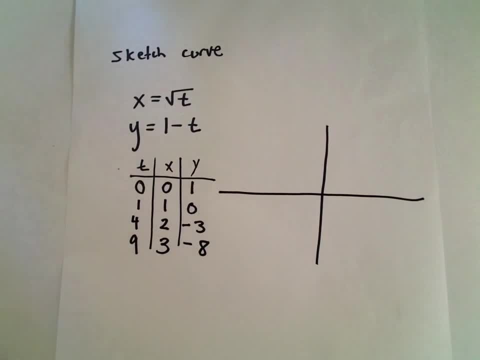 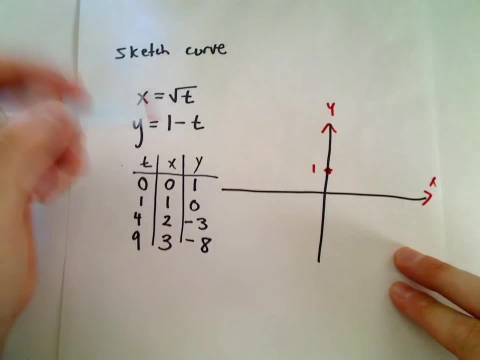 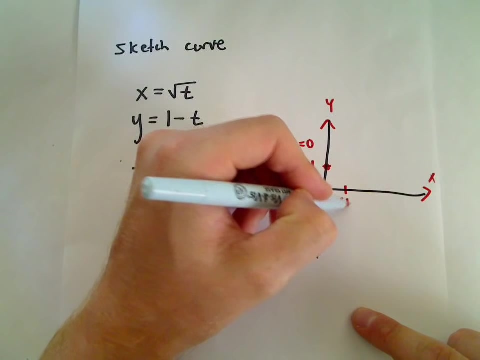 So at t equals 0,, we'll be at the point. Again, that'll be our initial point. So 0, 1.. And again, this corresponds to t equals 0.. At t equals 1,, we'll be at the point. 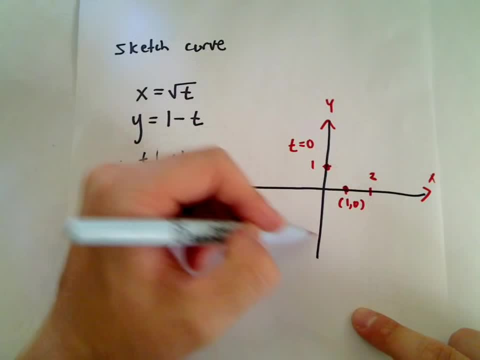 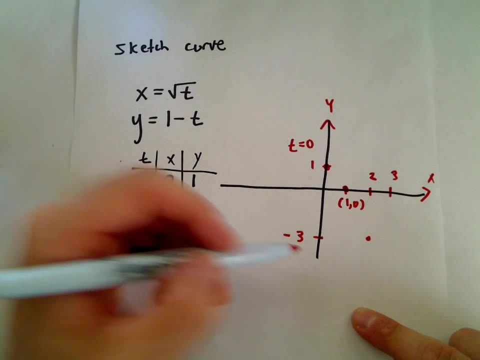 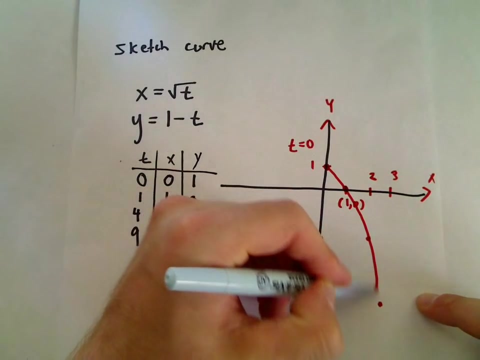 At: t equals 4, we'll be down here at And then at 9, we'll be at the x coordinate of 3 and the y coordinate of negative 8. So maybe we can just play connect the dots. It looks kind of like a part of a parabola which kind of makes sense. 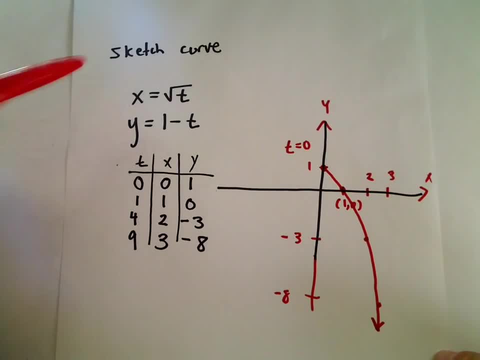 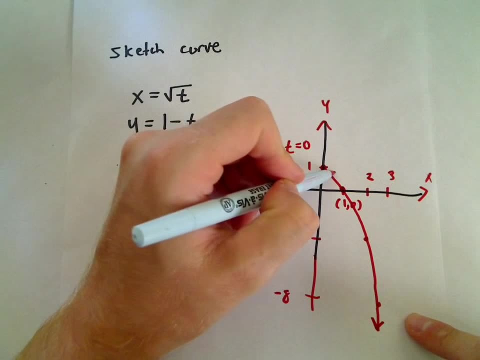 The x coordinate's getting bigger, The y coordinate's going to get more negative. This is another important part about parametric curves too. Parametric curves are curves that have a direction associated with them. So notice, as t increases, the coordinates would actually kind of move off to the right and down as your parameter t increases. 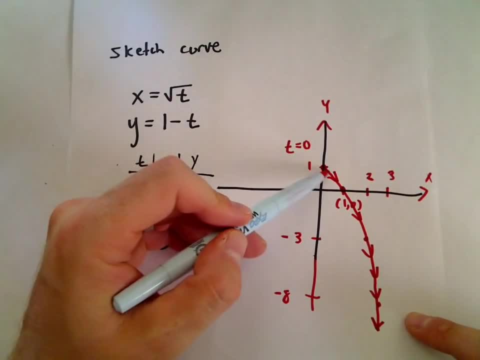 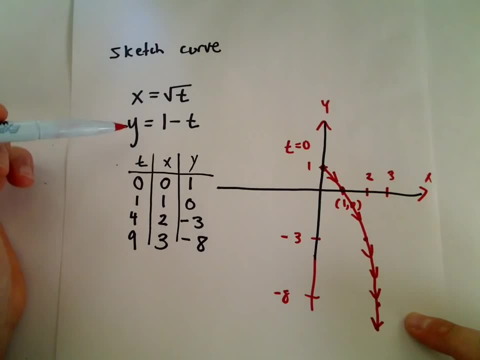 So the direction of this curve? the curve is moving The particle, if you want to think about this as a particle at any particular time, and x and y are formulas for its coordinates. Notice the curve is just moving down and to the right. 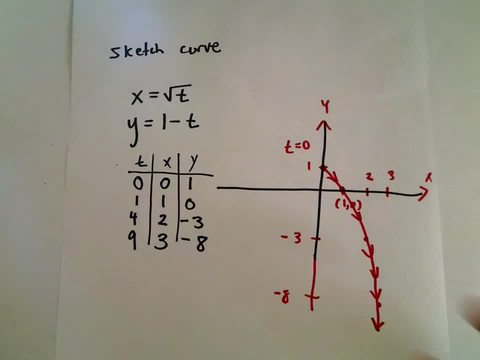 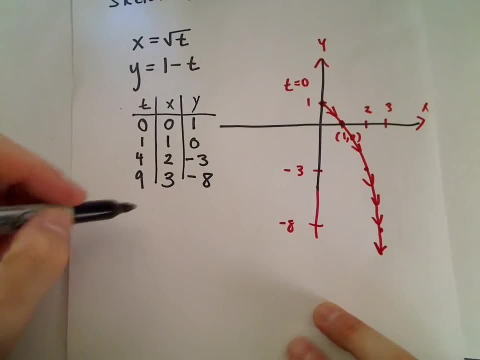 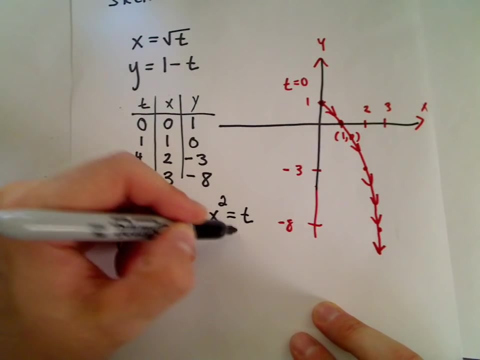 And this brings up one other little important idea. You can actually do what's called eliminating the parameter. Notice, we have x equals square root of t And y equals 1 minus t. Notice, if I solve, x equals square root of t. if I square both sides, I'll simply get that x squared equals t. 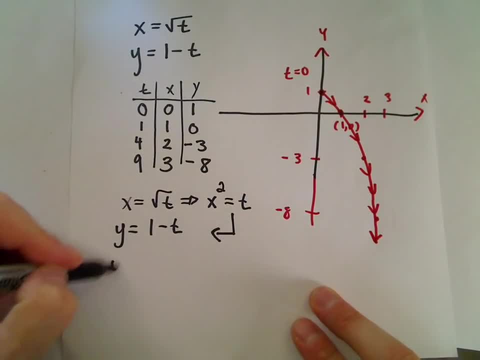 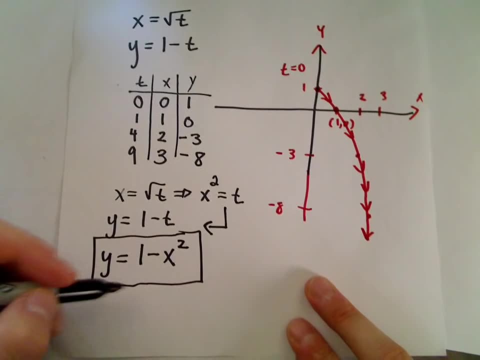 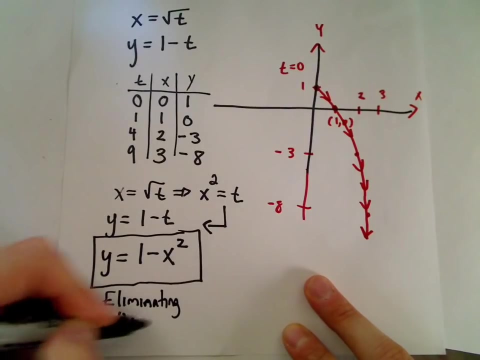 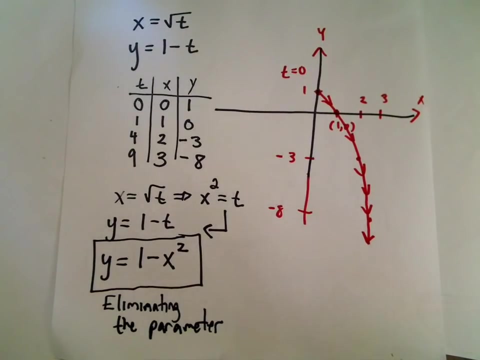 And then, if I substitute that into my other equation, I'll get that y equals 1 minus x squared, And this is now what's called eliminating the parameter. We have now eliminated the parameter t, So we've eliminated the parameter. And if you think about the graph of 1 minus x squared, well, what does 1 minus x squared look like? 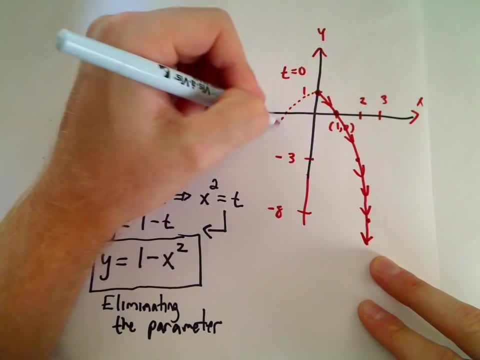 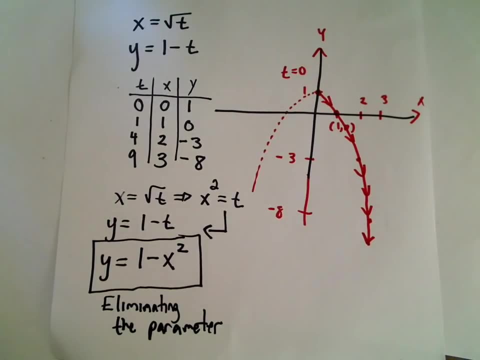 It's a parabola flipped upside down that has moved up one unit, So when you eliminate the parameter, you have to be careful though, because in this case our graph isn't the entire parabola, It's only the right-hand side of the parabola. 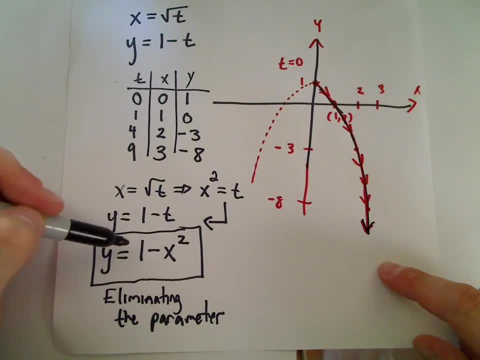 But once you've eliminated the parameter, it basically says your curve is going to at least be part of the graph that you've produced. So in this case I know that when I sketch, x equals square root of t, y equals 1 minus t. 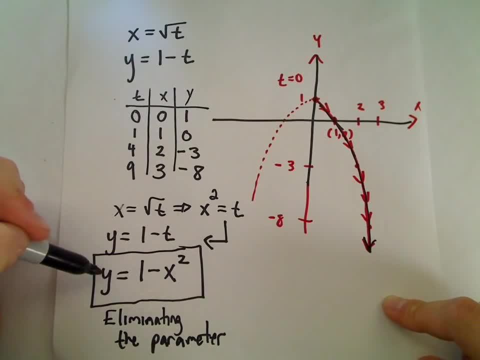 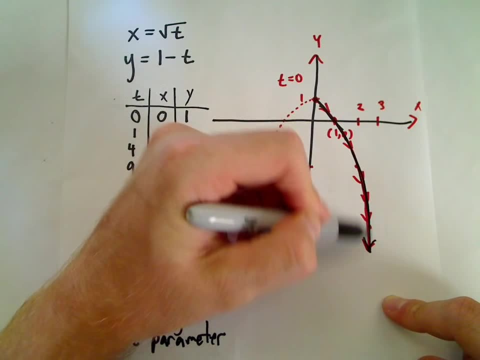 I know that the graph of that is going to look at least like a portion of the graph of 1 minus x squared, And in fact that's what's happening. So to kind of determine what part of the graph you get, then you have to go back and think about domains on t. 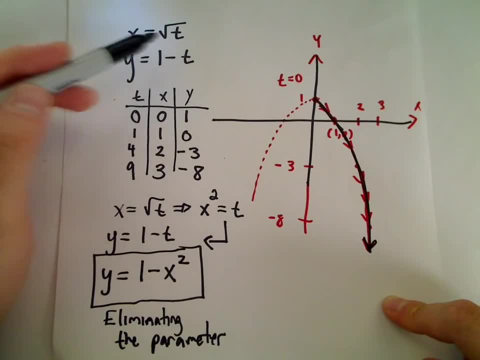 The domain of your x and y coordinates, what t values are acceptable to use, And from that you'll often be able to deduce what portion of the graph you're getting. So here's some little basics on herometric equations. I'll do some more graphing and also talk about tangent lines and more complicated things in another video. 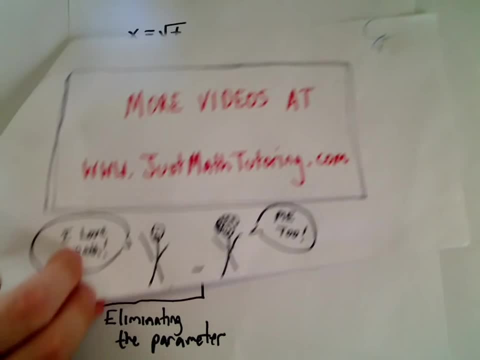 Feel free to look around YouTube. I will also have links to all of these on my website, Along with a lot of other videos, So feel free to take a look there too.